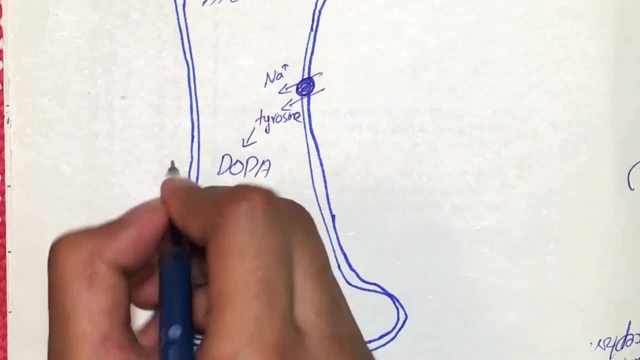 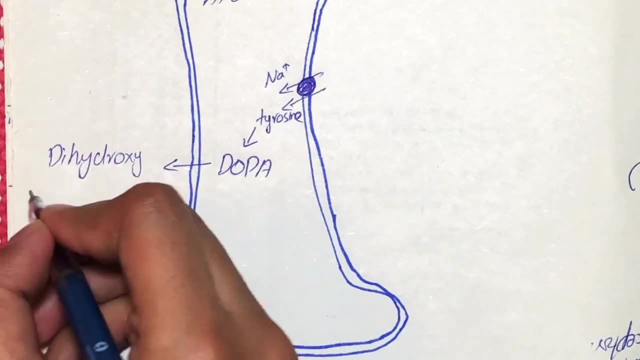 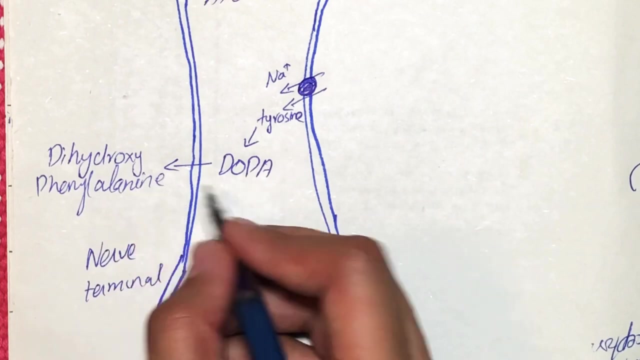 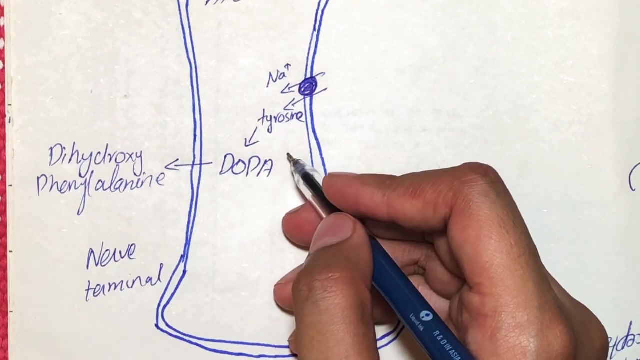 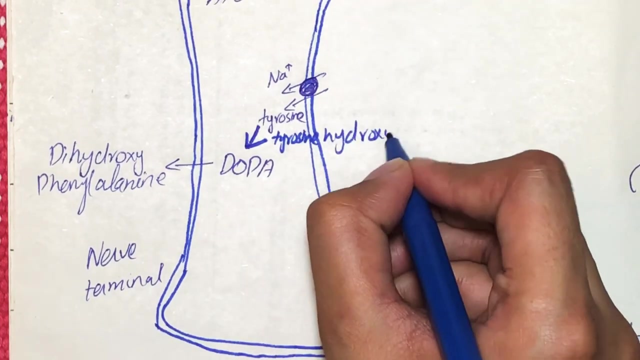 DOPA, And DOPA is what stands for dihydroxyphenylalanine. This is what DOPA is. So tyrosine is converted into DOPA by the action of an enzyme called as tyrosine hydroxylase. So this enzyme converts. 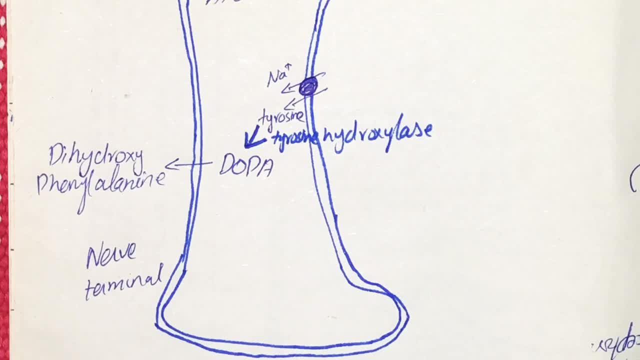 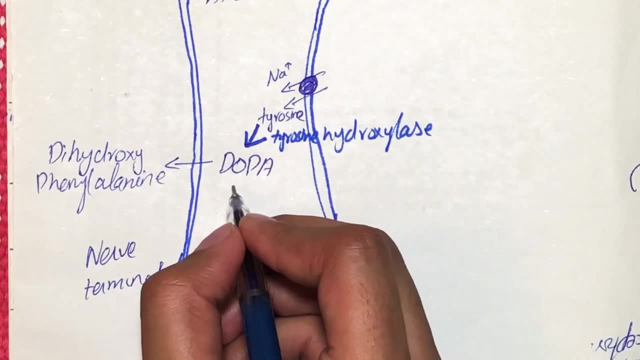 the tyrosine into DOPA, which is dihydroxyphenylalanine. So, after the formation of DOPA in the cytoplasm of the cell, what happens is that this DOPA is then converted into dopamine And this 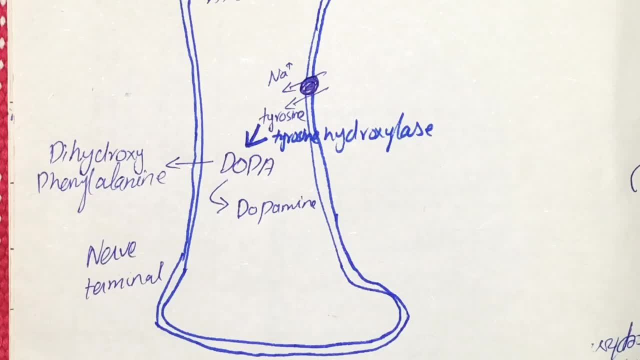 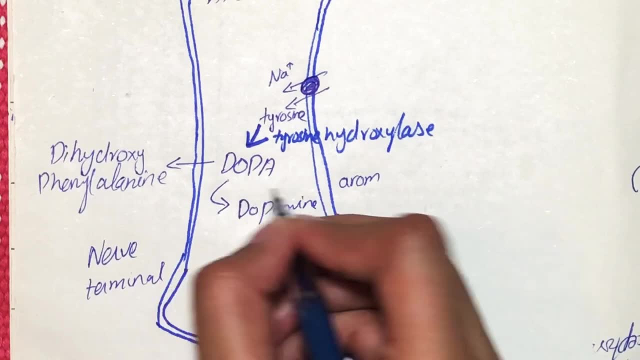 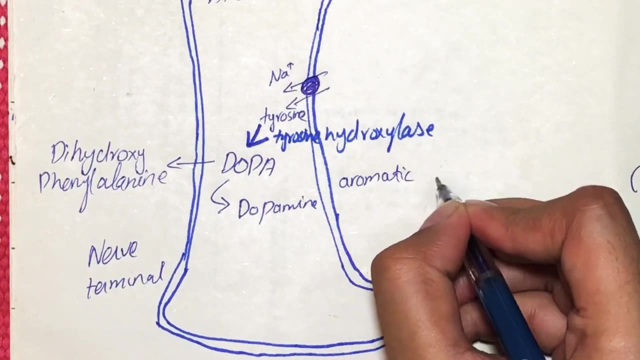 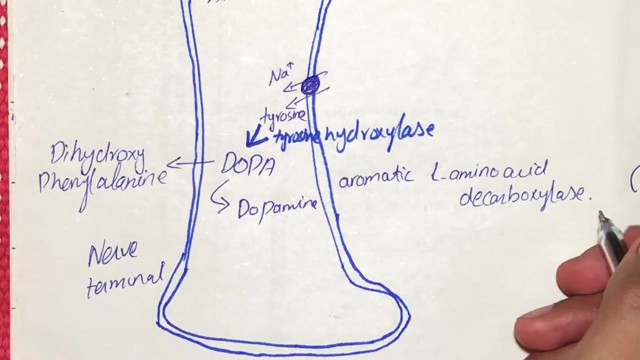 is also done by the action of an enzyme called- as I'm writing it here. the enzyme that is acting is inside the cytoplasm, but because I have no place here, so I'm writing it here- Aromatic L-amino acid d-carboxylase, So this enzyme acts over here in the cytoplasm. 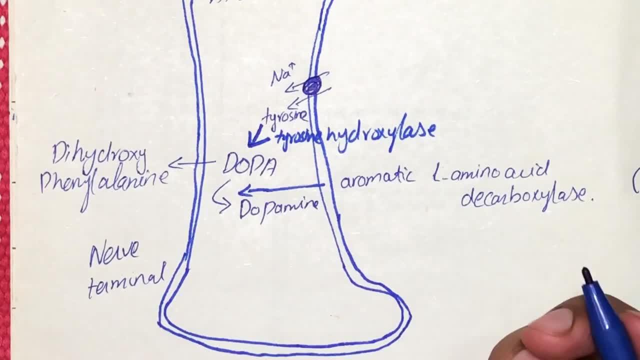 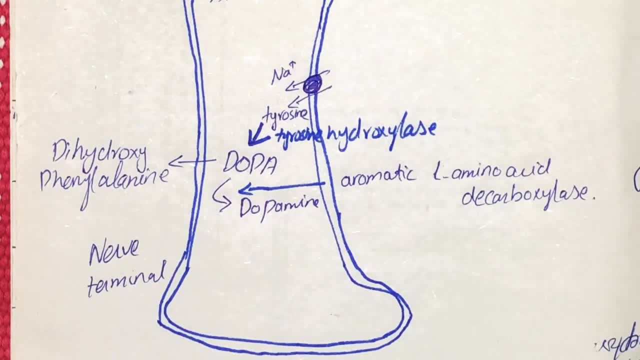 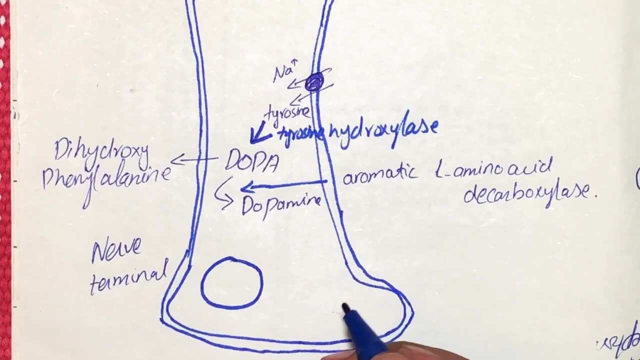 And this is what I'm writing here again. So this enzyme acts over here in the cytoplasm and that site appears to be different. If I'm writing here, if I'm writing here, if it appears to be 1,037, then I'm writing it back down to a 4-1-1,0100.. From there I'm going. 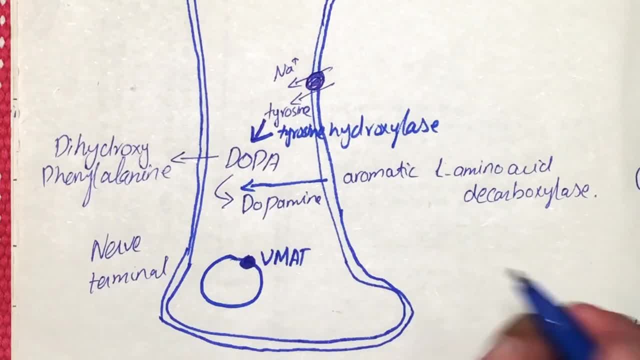 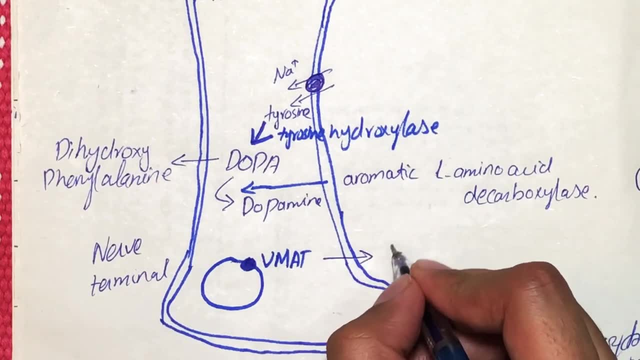 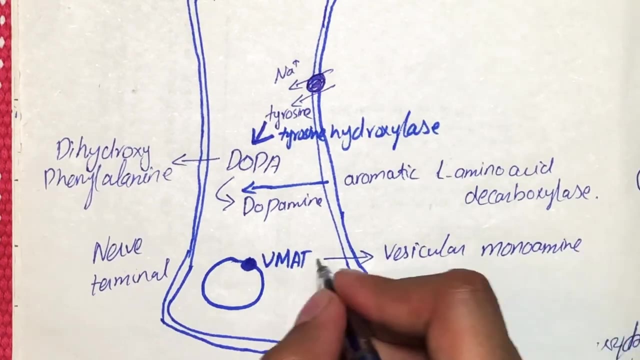 to write the 0, and now I'm writing this down to 0 and back it down to a 3. Let me write away if Ifer 7. transporter, So let me write it here for you: Vesicular monoamine transporter. So its short. 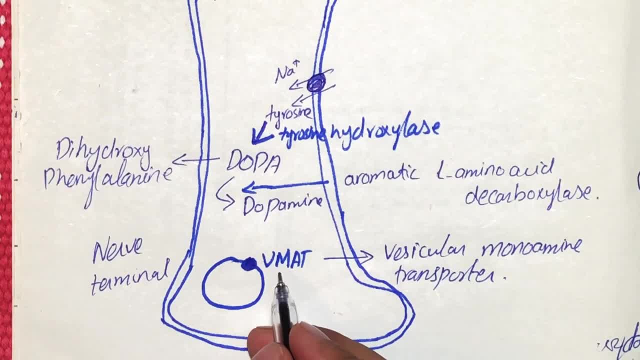 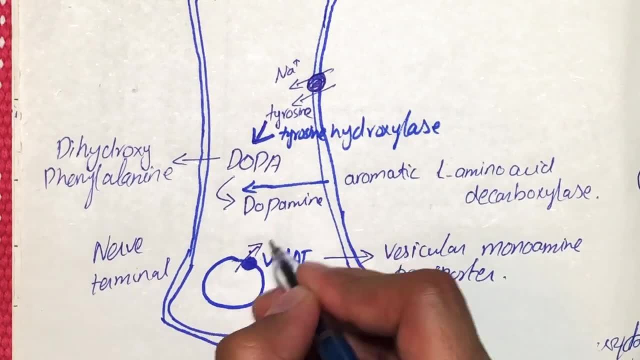 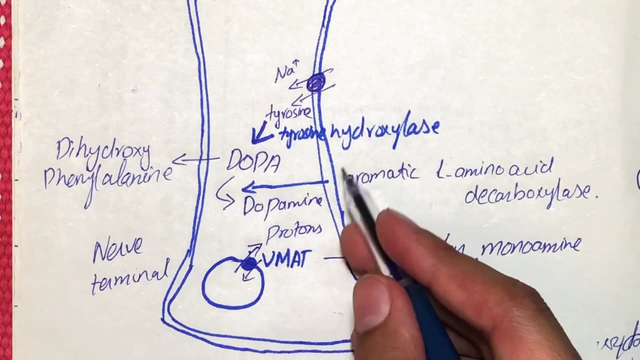 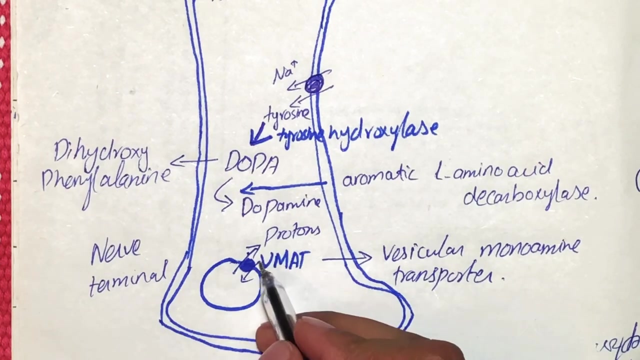 form is VMAT. So what happens is this VMAT is an antiporter, and what this antiporter do is it caused the influx of protons and influx of dopamine present in the cytoplasm of this neuron. What VMAT do is that it caused the exchange of two molecules, or two things, which 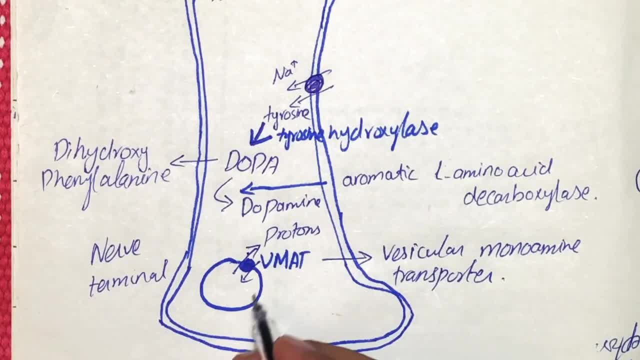 are protons and dopamine. So after the exchange of these two we have dopamine inside the vesicle and dopamine is then converted into dopamine norepinephrine by an action of enzyme present inside the vesicle, which is- i'm writing it here- 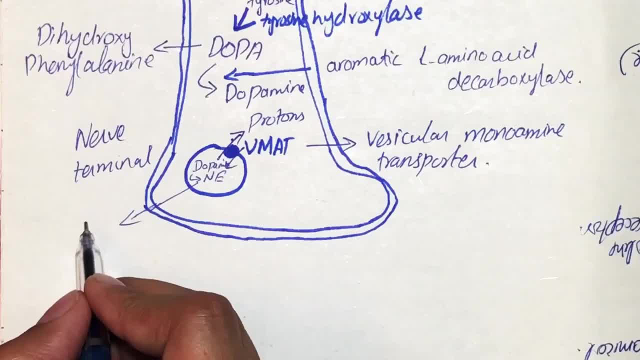 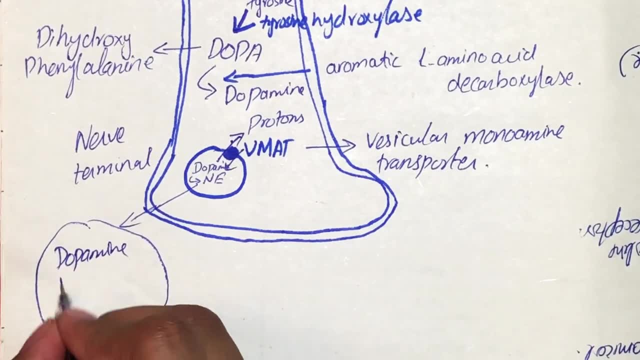 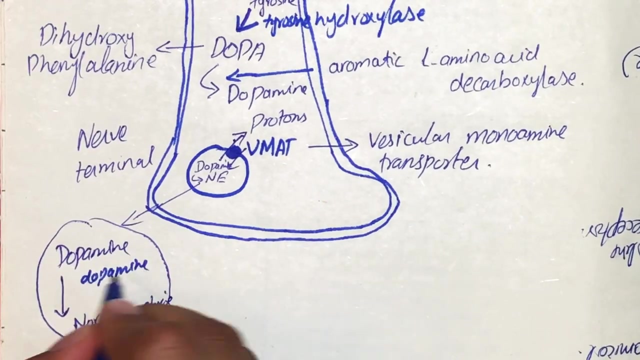 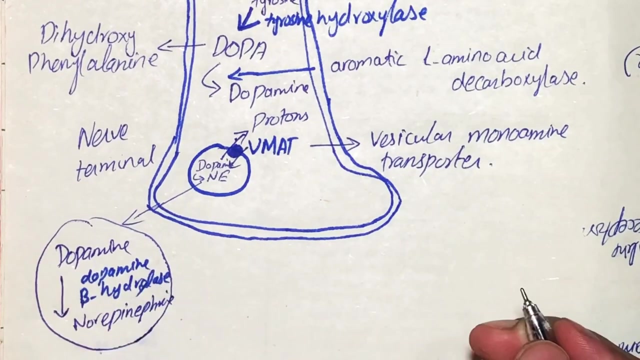 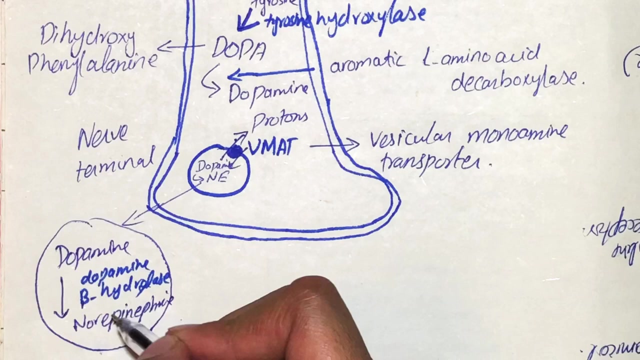 again because i have less space. so if it is our vesicle, we have dopamine in it. so dopamine will convert into norepinephrine by an action of enzyme or as dopamine beta hydroxylase. so this enzyme is present inside the vesicle, not in the cytoplasm. therefore, after being packed, 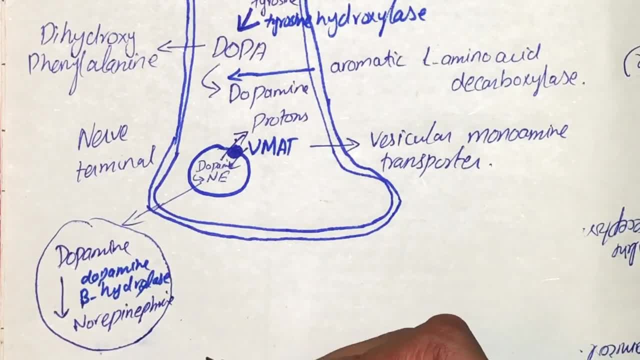 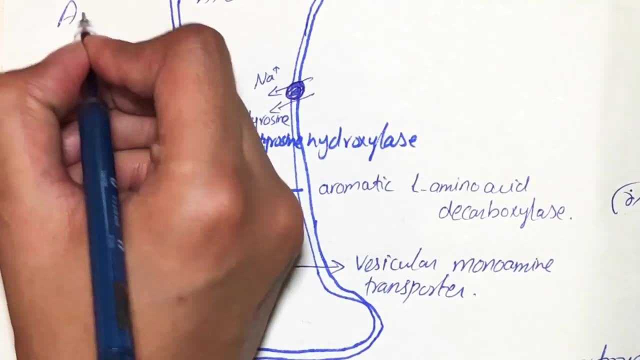 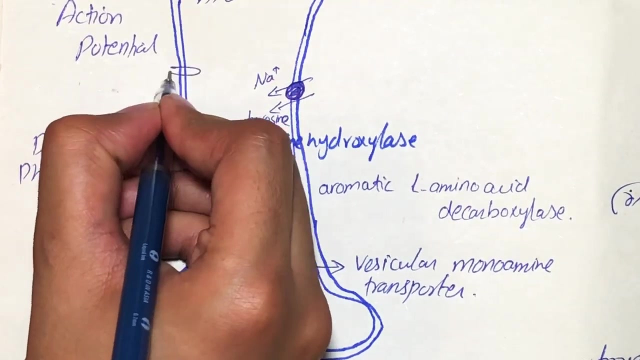 in the vesicle. dopamine is then converted into norepinephrine through the action of this enzyme called as dopamine beta hydroxylase. so now we have norepinephrine inside the vesicle. so now what happens when action potential arrives? there is an influx of calcium ions into the 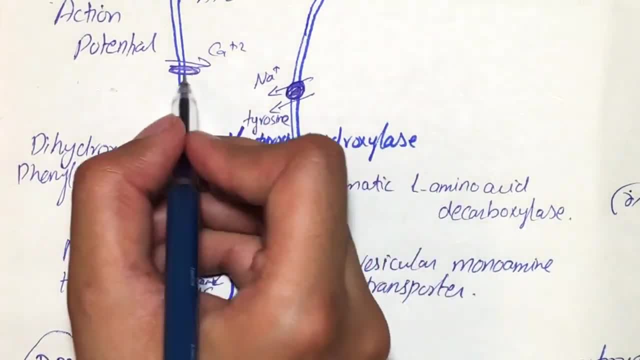 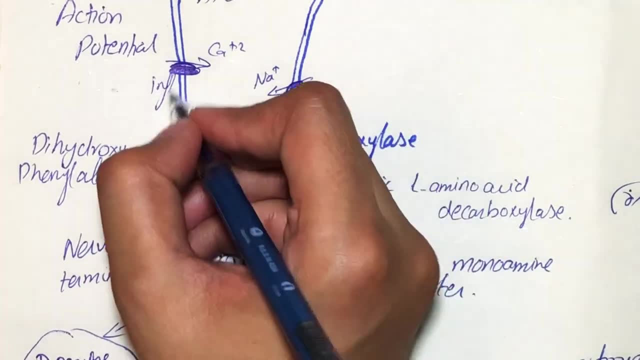 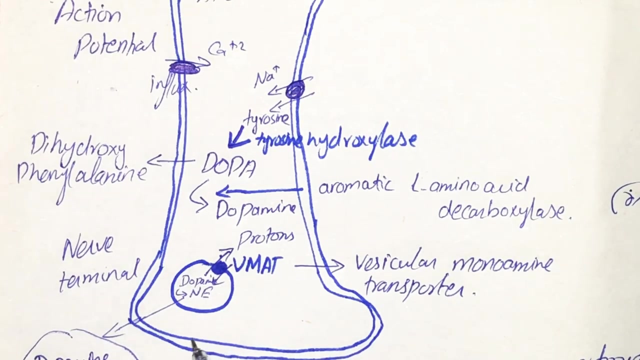 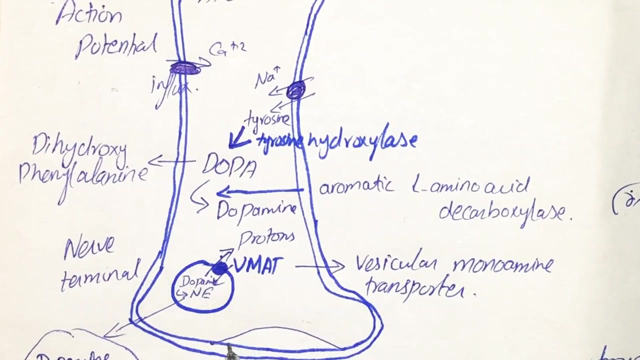 cytoplasm of the neuron through the calcium channel. so, after the influx of calcium ion, what happens? What happens is that these vesicles, which are previously formed and have norepinephrine in them as primary neurotransmitter, these vesicles diffuse into the membrane of the 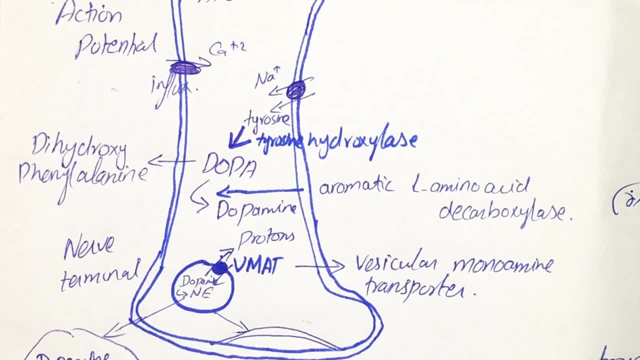 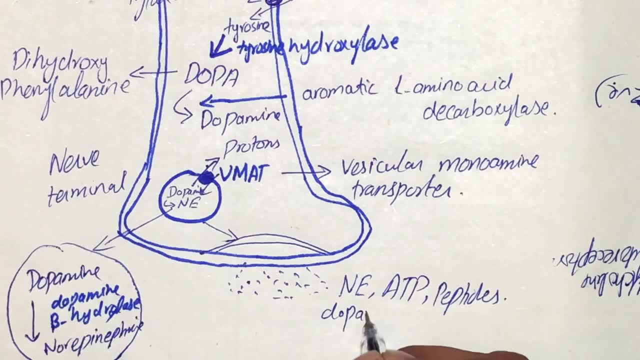 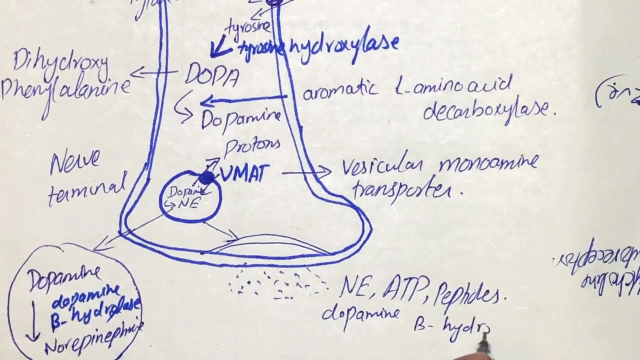 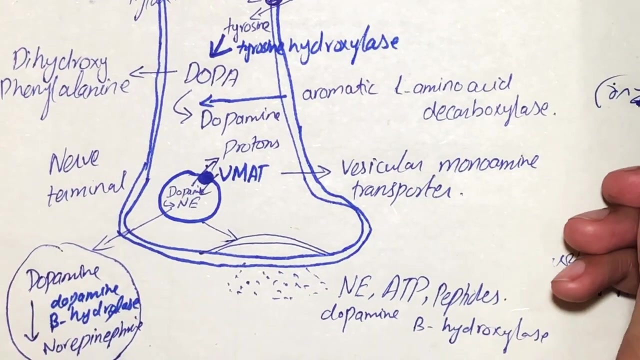 neuron and thus cause the release of neurotransmitters. So primary neurotransmitter here is norepinephrine, while other substances like ATP, peptides and dopamine beta-hydroxylase, which is the enzyme that causes the formation of norepinephrine, is also present in synaptic left after the fusion of synaptic vesicle into the presynaptic. 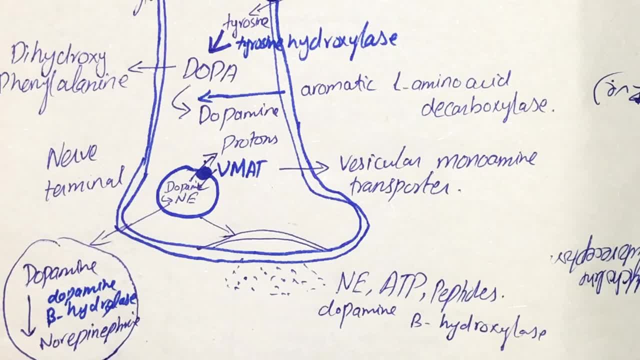 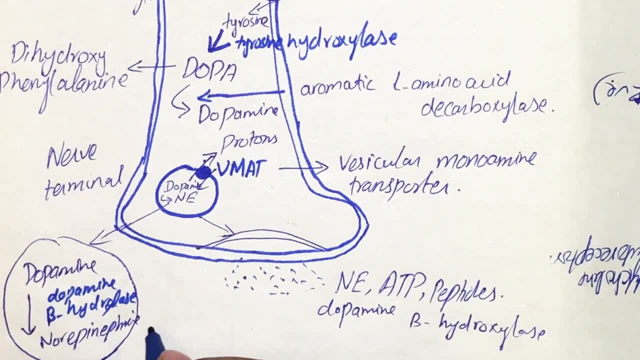 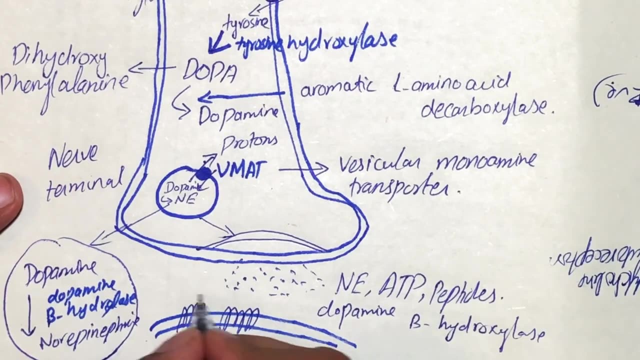 membrane. So after the release of norepinephrine in the synaptic space, we can have three different possibilities. if this is the postsynaptic membrane, We have adenoceptors on the postsynaptic membrane. We have adenoceptors on the synaptic membrane on which, when norepinephrine bind and cause. 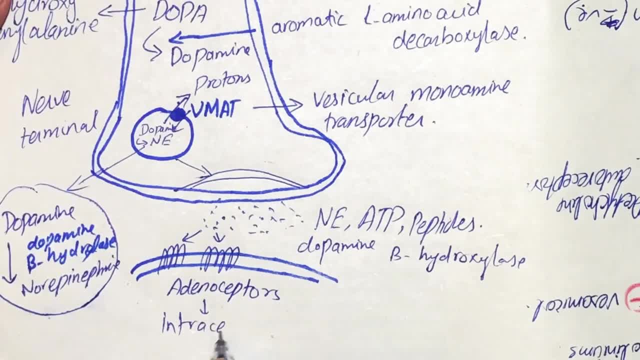 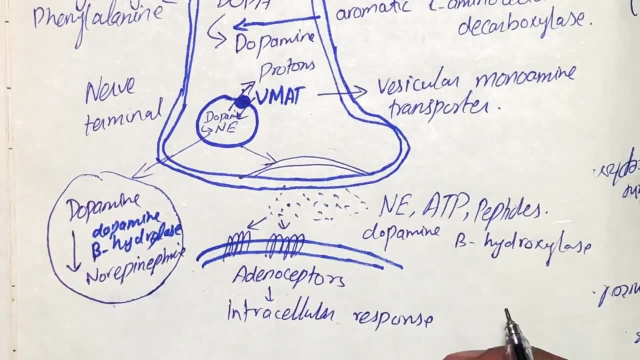 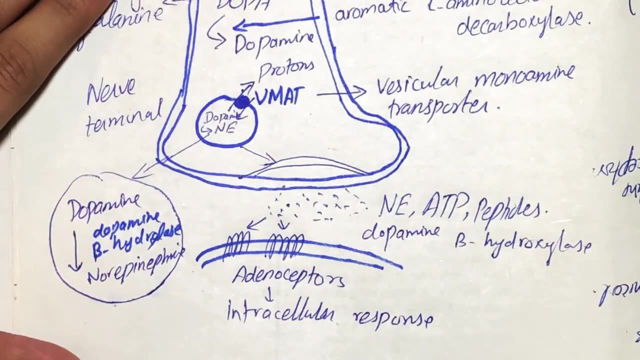 the intracellular response. So this can be the first possibility for the norepinephrine present in the synaptic left. What can be the second one? We can have a transporter called as Norepinephrine. What is a transporter? Transporter is a transporter of Norepinephrine. 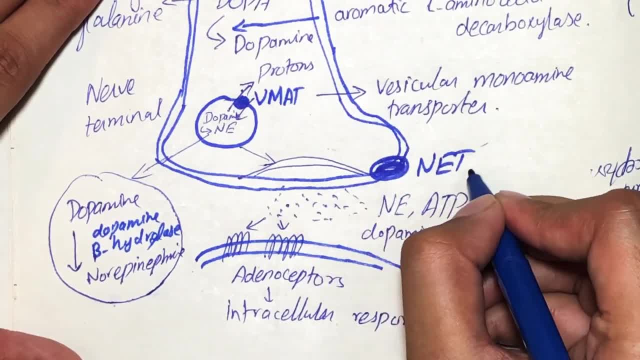 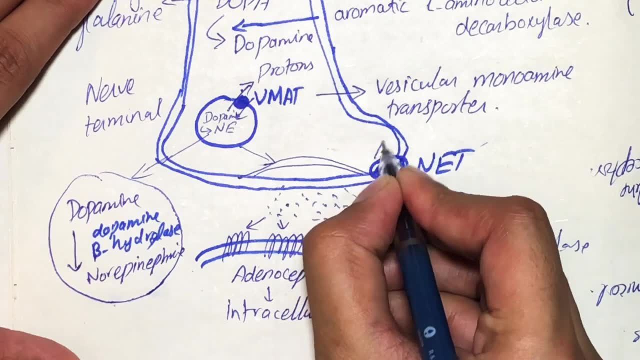 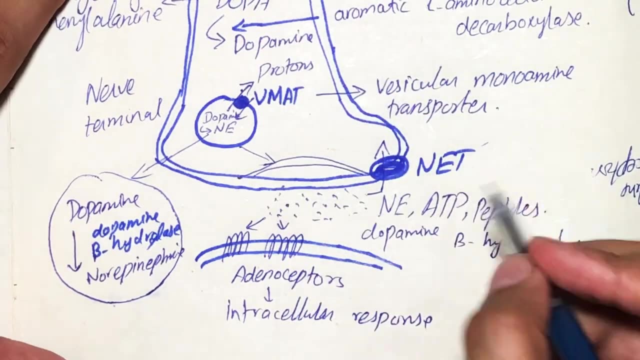 It is a transporter of Norepinephrine. It is a transporter of Norepinephrine which is not epinephrine transporter. What this transporter do is that it takes back the norepinephrine present in the synaptic left into the cytoplasm of presynaptic neuron. 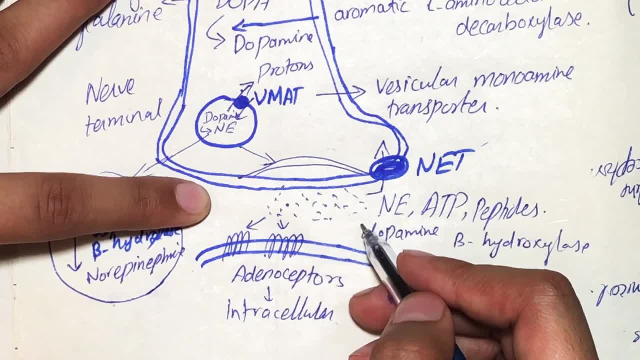 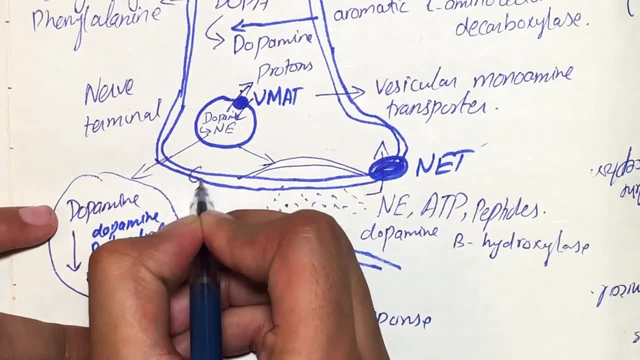 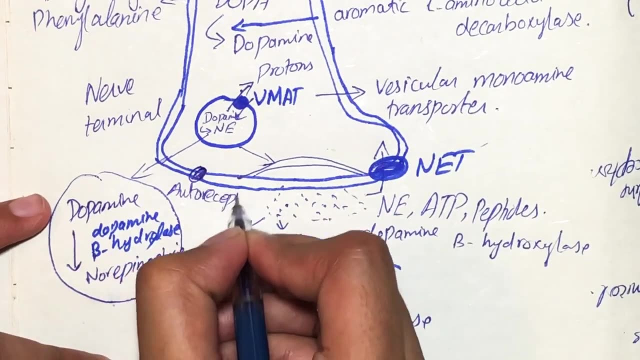 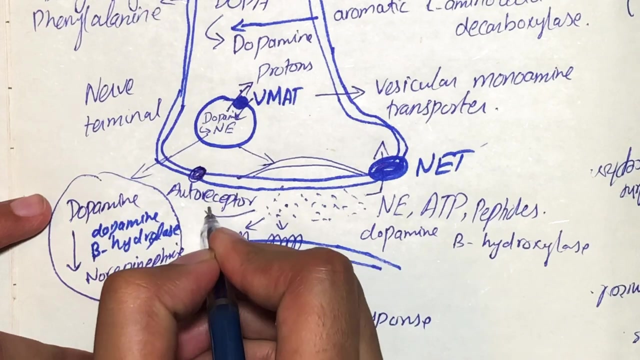 So in this way, less of the norepinephrine is present in the synaptic left for the cellular response. And what could be the third possibility? It can have autoreceptors, receptor on presynaptic membrane of the neuron which can cause the shutdown of further release. 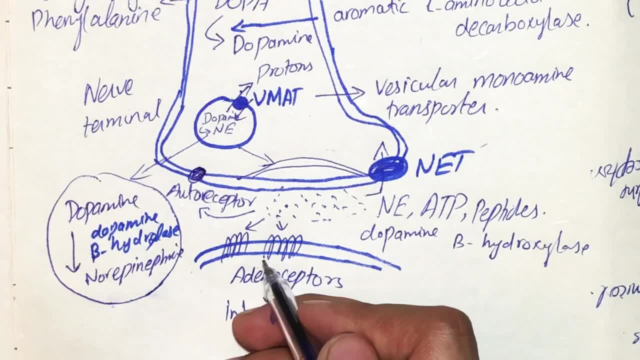 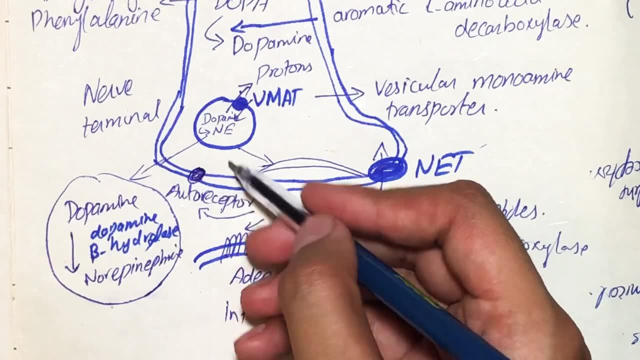 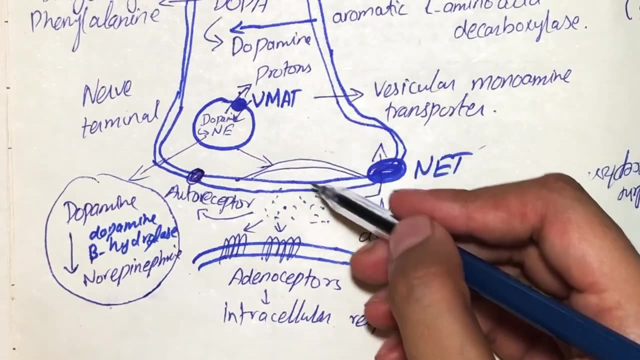 of norepinephrine vesicles. It is like shutdown button for the norepinephrine release. when this shutdown button is being turned on, what actually happen is that no further vesicle diffuse to the presynaptic membrane and therefore no further release of norepinephrine occurs. 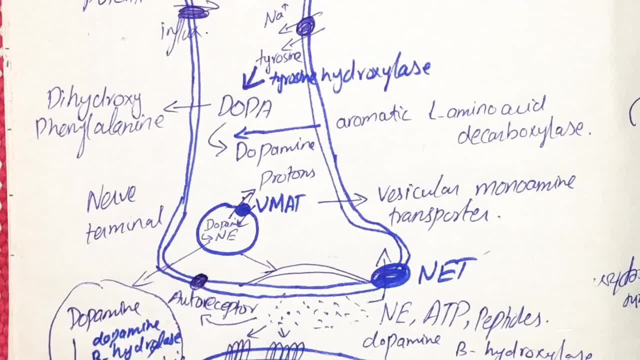 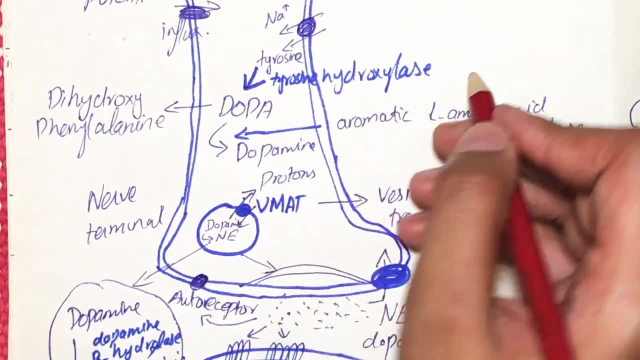 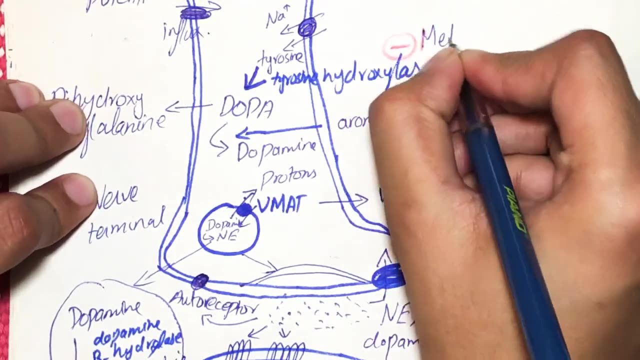 So in this way these three possibility can occur. So we have different drugs acting on these enzymes or transporters. So for tyrosine hydroxylase we have a drug which inhibit the action of this enzyme and it is called as methyrosine.